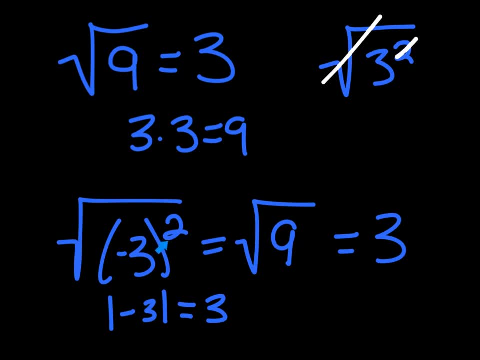 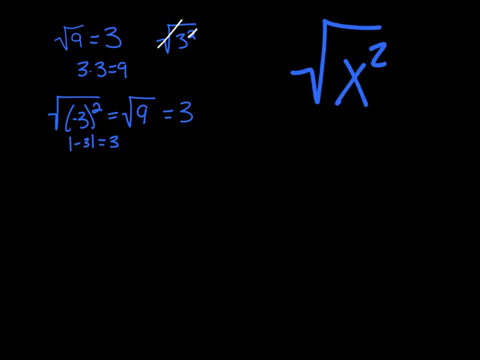 even exponent. we know that this even exponent inside ensures that the whole radicand become positive first before applying the radical, and therefore we always need to take the absolute value. Therefore, if we're taking the square root of x squared, even though in our head 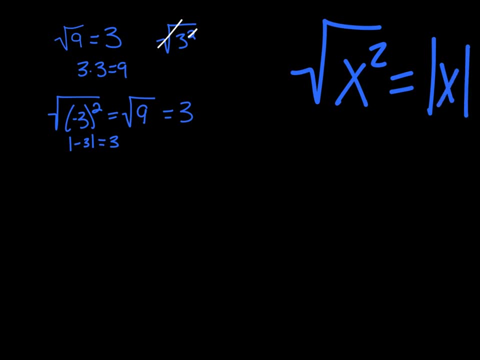 we may think it's x, it's really the absolute value of x. So, more generally, if we have an even index and an even exponent inside and it results in an odd exponent, then we put absolute value bars around the x. This rule gets more complicated, but this: 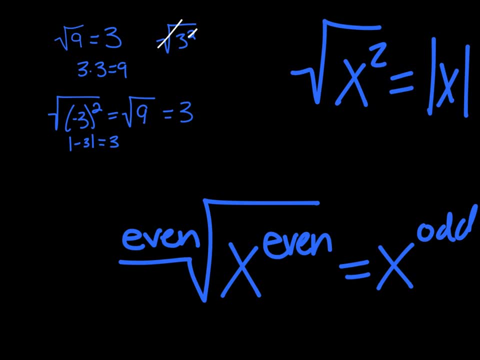 is a good basic rule to follow. The reason why we only need these if our exponent on the outside is odd is that if we had an even exponent, we already would be ensuring that we have a positive answer, But if we have an odd exponent we could end up with a negative. 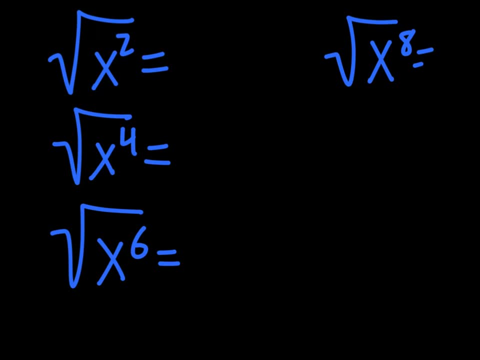 outside. So when we take the square root of x squared, the result is the absolute value of x. When we take the square root of x to the fourth, the result is just x squared, because this squared already ensures our positive answer. When we have the square root of x to the sixth, 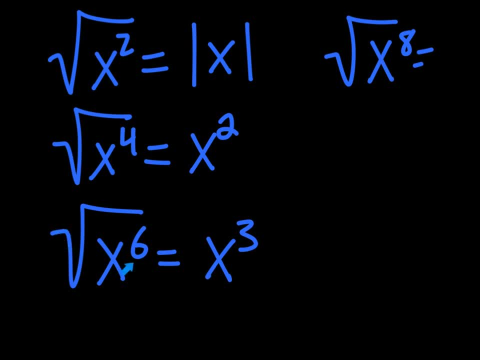 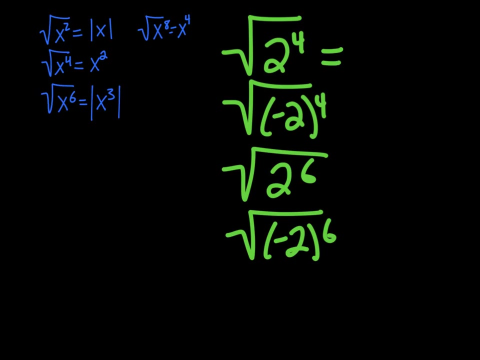 we get x to the third, but we had even, even odd, so therefore we do need our absolute value bars. The square root of x to the eighth. you guessed it is just x to the fourth. If we looked with numbers, we would know that the answer to this is the square root of sixteen. 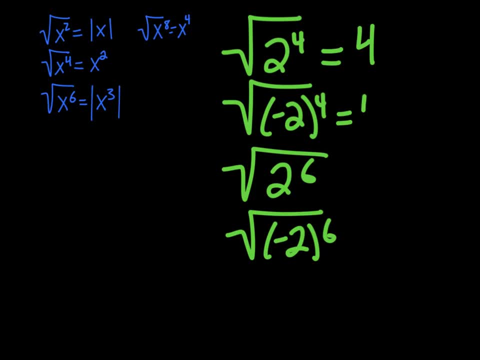 which is four. The answer to this is also the square root of sixteen, which is four. The answer to this is the square root of sixty-four, which is eight, And the answer to this is also the square root of sixty-four, which is eight. Notice that they're all positive. 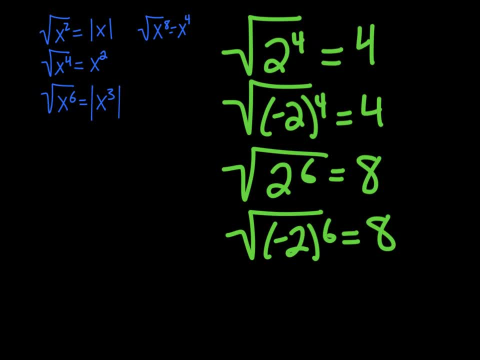 So really, we took the absolute value of each of our answers, even if there was a negative. to start with Subtitles by the Amaraorg community. We only write the absolute value- bars if we're dealing with a variable, not a number. 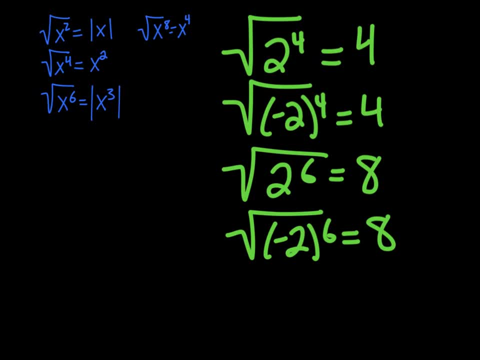 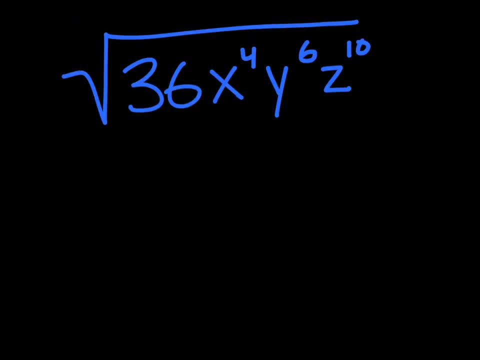 For example, we would write positive eight instead of the absolute value of negative eight. if that were the case, Here's one final example. The square root of thirty-six is six. That's already positive. If we had a negative, we would have an imaginary solution. The square root of x.